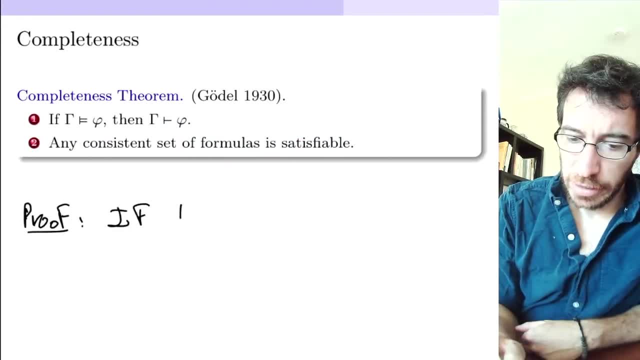 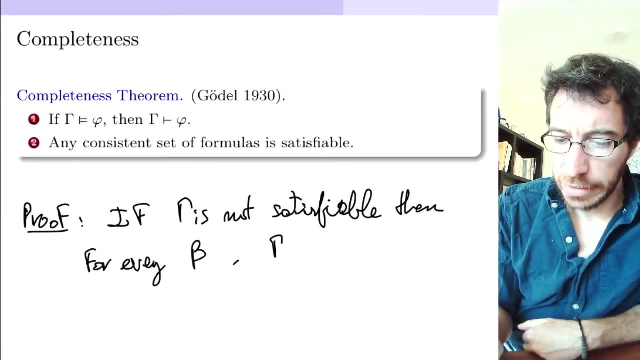 The proof of this is that if gamma is not satisfiable, then for every formula, beta gamma semantically implies beta. The reason for that is that if you're not satisfiable, you don't have any model. So it's trivially true that every model of gamma is a model of beta. 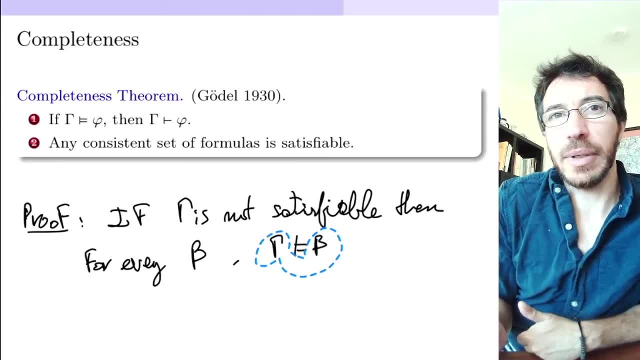 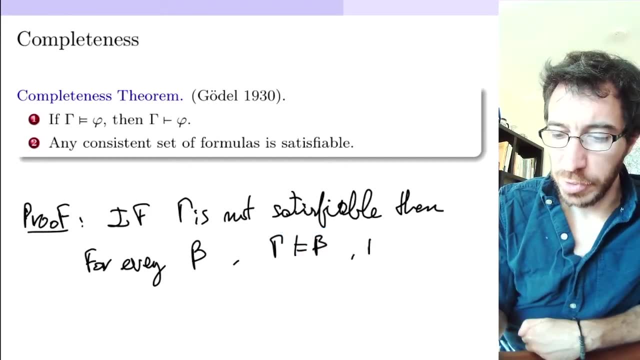 Every model of gamma is a model of beta, Just because there are no models of gamma. So this is true for every formula. It will be implied, and also then that means that you will get also the negation. That will also be implied. 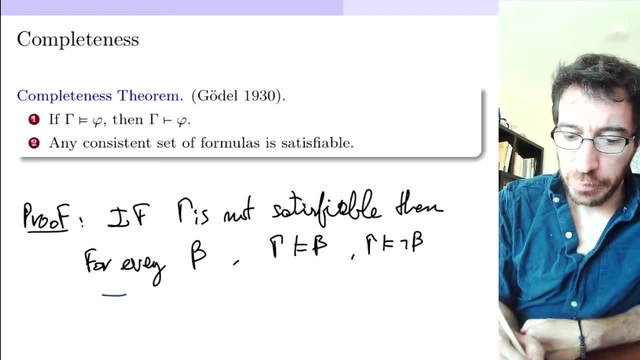 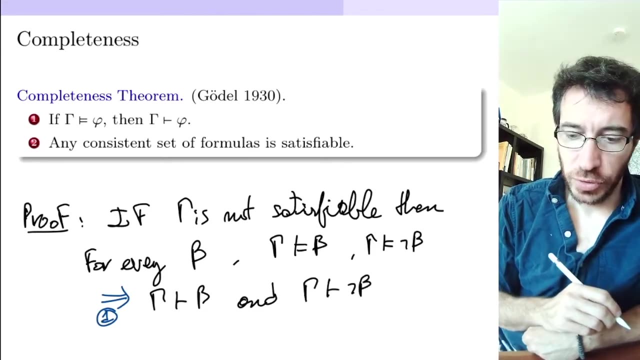 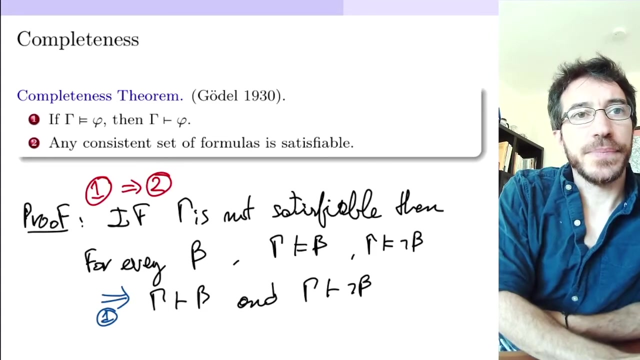 But then by the completeness theorem, by part one, you will get that gamma proves beta and gamma proves not beta. So that's how you, how you get that one implies two, Which you haven't provided. What's the reason that two implies one? 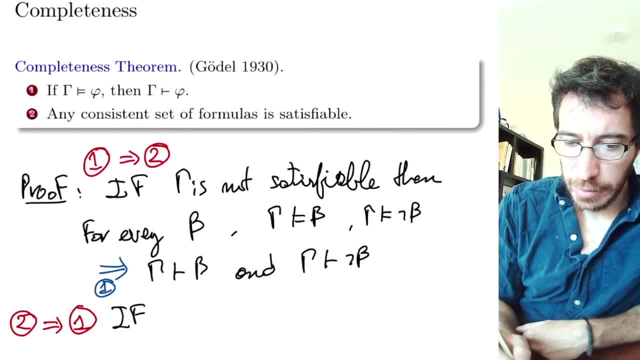 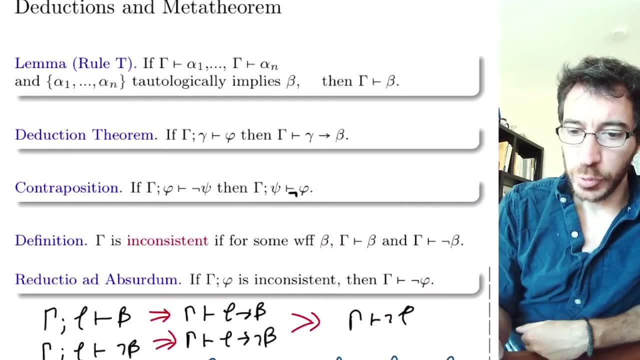 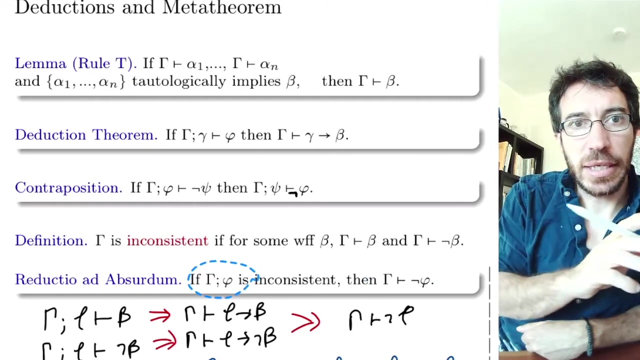 And this is by a contrapositive: If gamma does not prove phi, then by the reduction to absurdum that we proved last week. if you don't prove something, then gamma and the negation are consistent. Okay, so we're going to use this one in the opposite direction. 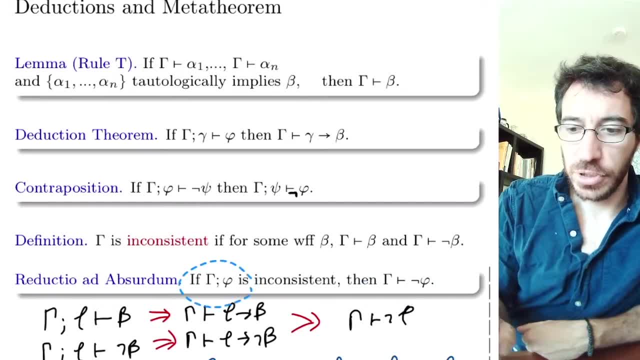 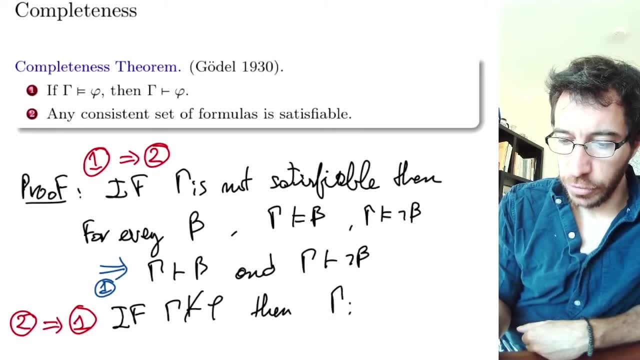 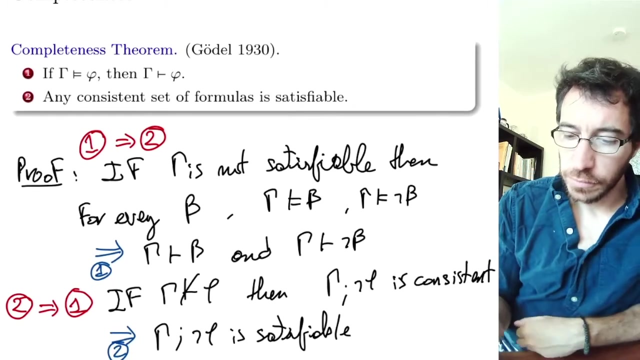 If you don't prove, then this is not inconsistent. So if you don't prove phi, then gamma together with not phi is consistent, But then by part two gamma together with not phi is satisfiable. But then that implies that gamma does not logically imply phi. 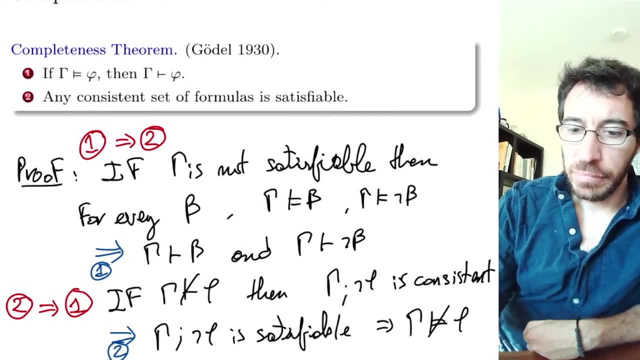 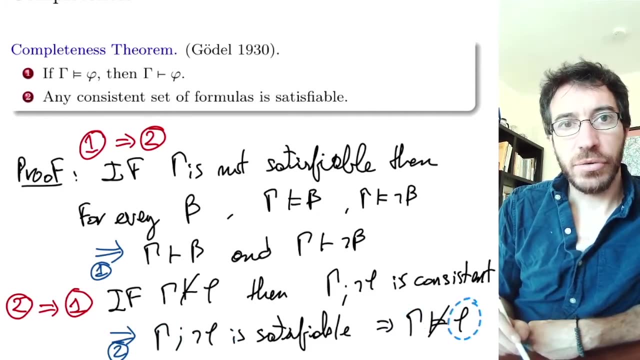 Because gamma logically implies phi means that every model of gamma is a model of phi And this, being satisfiable, says that there exists a model of gamma which is not a model of phi. So that means gamma cannot imply phi And that's what we get from this. 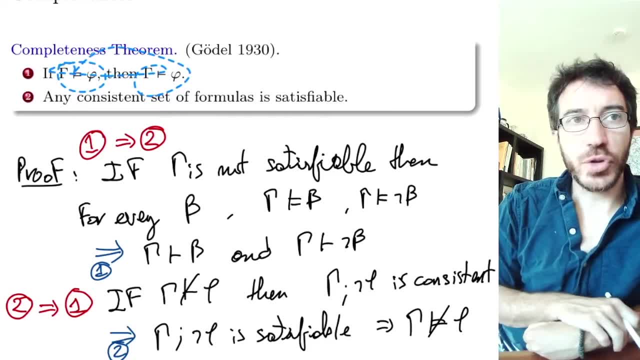 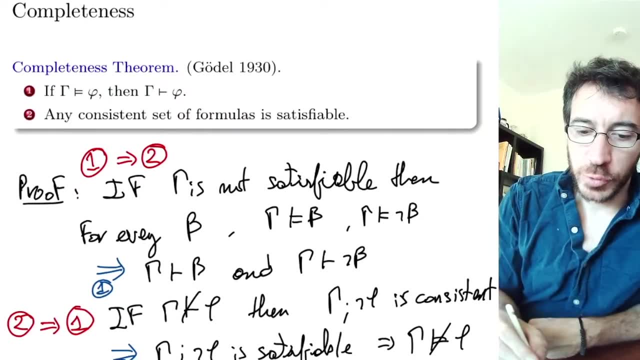 Contrapositive Cool. So those two are equivalent and together they are called completeness theorem. We're actually going to prove this one. We're going to show that if you're consistent, then you're satisfiable, and that's going to imply the other one. 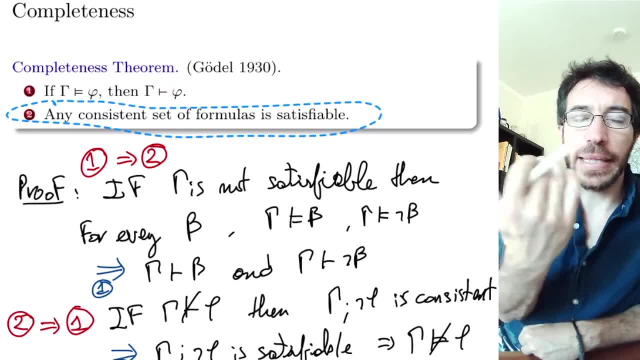 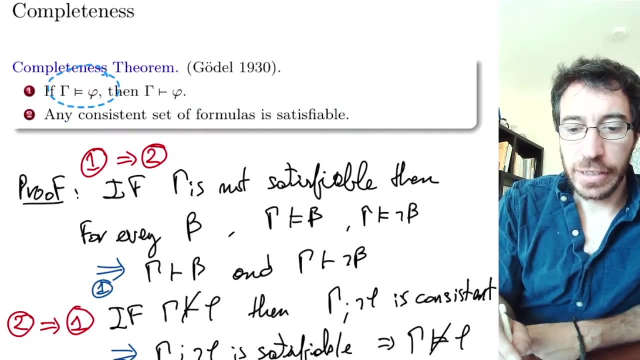 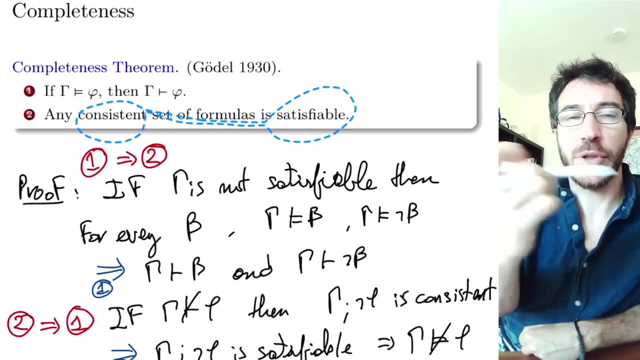 Okay, and then this is actually going to get this together with soundness. We get if and only if. Essentially, we get that logical implication is equivalent to syntactical implication And we get that consistency is equivalent to satisfiability, using soundness for the other direction. 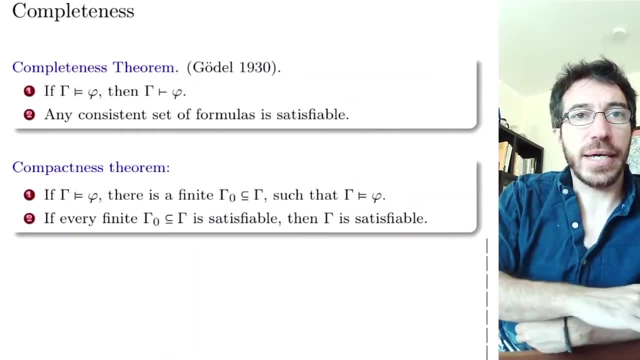 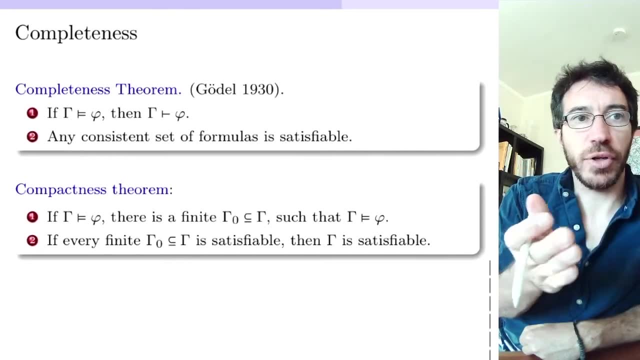 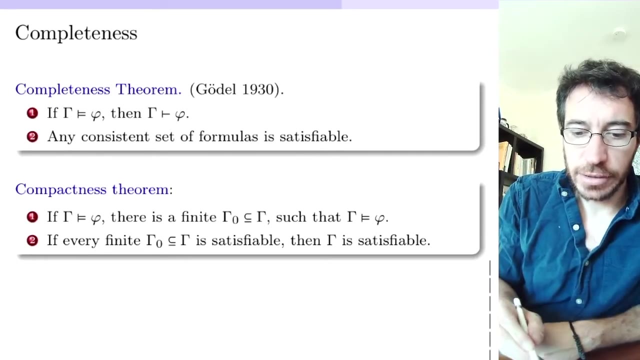 Okay, so one corollary of this that we've been using for a long time is compactness, So the compactness theorem follows directly from here. The compactness theorem has two versions, also like this one too, which we saw already that they are equivalent. 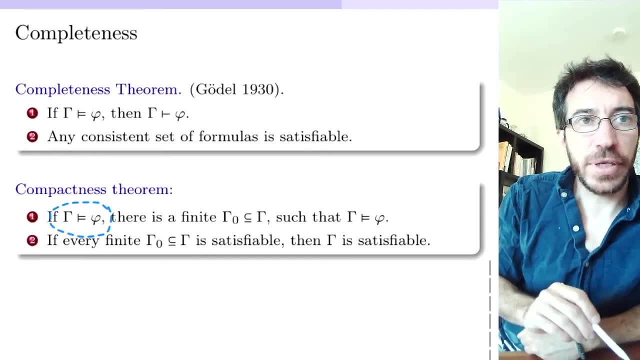 The first one says that if gamma logically implies phi, then there's a finite subset of gamma that already logically implies phi, And equivalently we say that this is the same thing as saying that if every finite subset of a gamma is satisfiable, 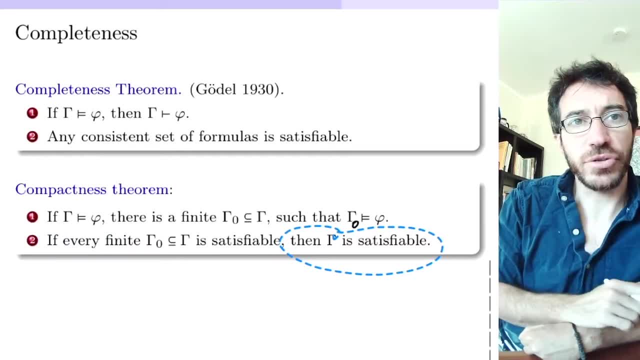 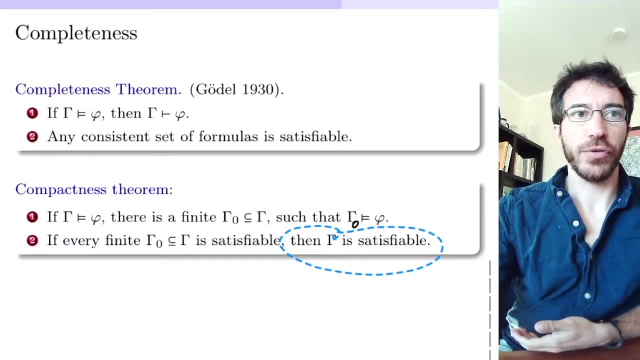 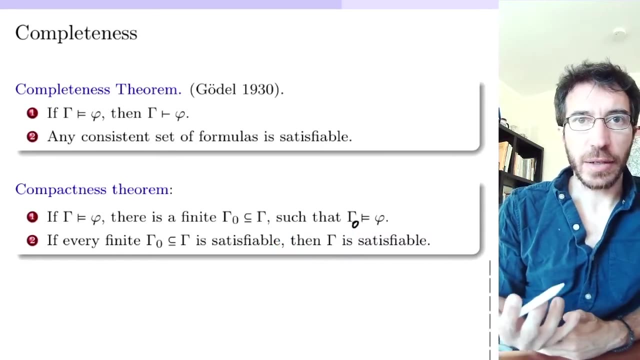 then the whole gamma is satisfiable Right. so we use both versions. Both are equivalent. We even prove that they are equivalent. So that's compactness. And why does it follow from completeness? Well, it's very simple, because by completeness and soundness together, 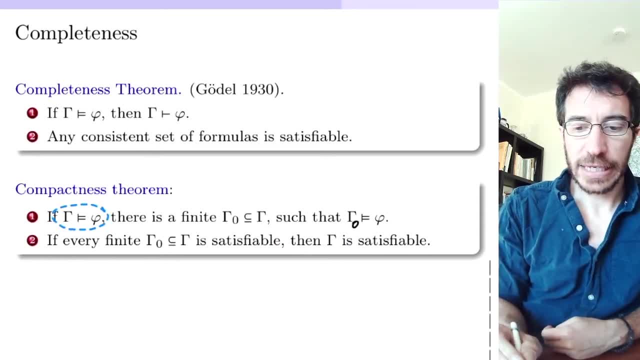 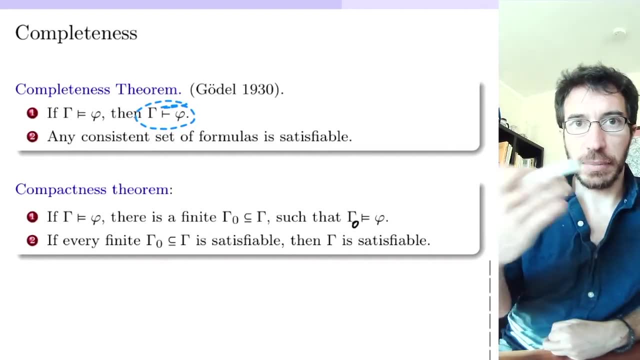 we know that logical implication is the same as a formal syntactic implication, right, And so they're back and forth, they are the same. So if a whole set of sentences proves this sentence, phi, that means we have a deduction, a formal deduction, of phi from gamma. 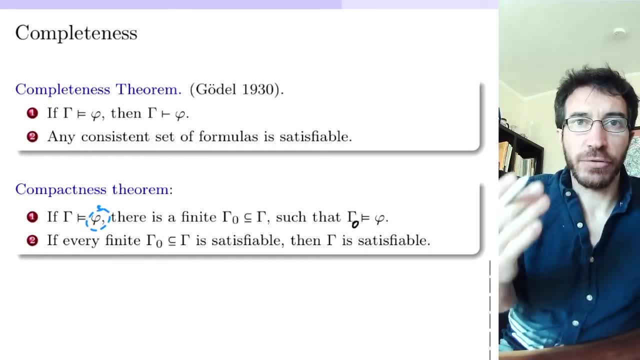 In the formal deduction we can only use finitely many sentences, right? A formal deduction is a finite list of formulas and some of those are used as assumptions, but only finitely many. So we are using finitely many of the assumptions in the proof. 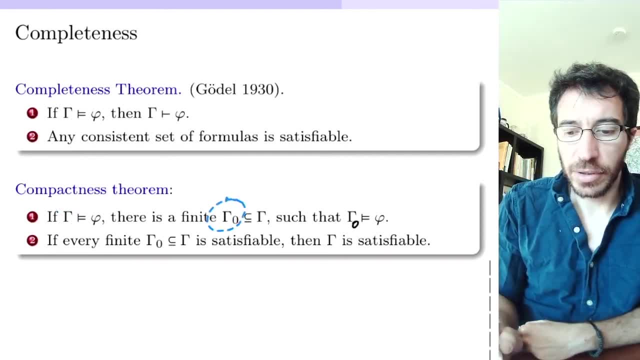 not more than that. So we can take a finite subset, which are the ones that are used in the proof, and that's enough to prove phi, which, again, if you prove phi, then by soundness you logically imply phi. So that's it. 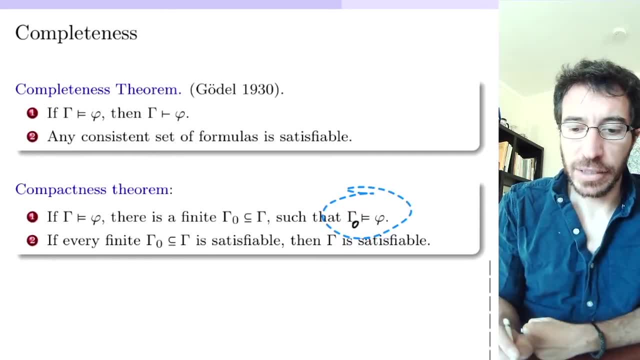 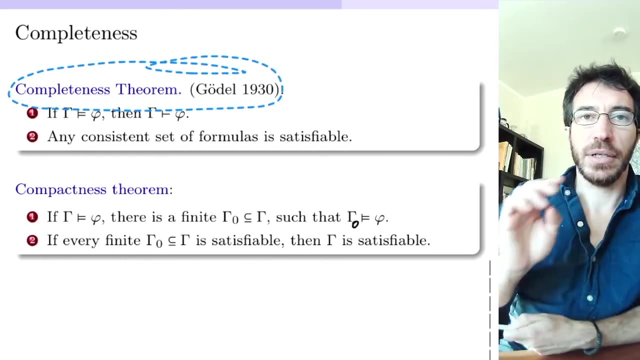 So that's the proof of compactness. So compactness is very easy. if you look at formal deductions, and completeness and soundness tell you that formal deductions are the same as logical deductions. Okay, so we'll actually do this proof in the next coming weeks.